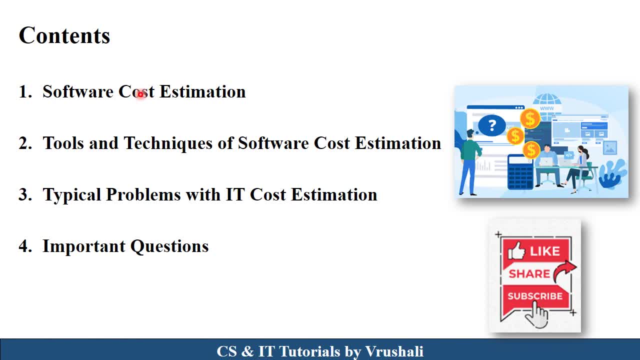 the session. In this session we will discuss about software cost estimation. their tools, techniques and different problems occur in cost estimation. At the end we will discuss some important questions that have asked in previous year question paper. Let's see all these points one by one Now. the first thing is: what exactly software cost estimation? 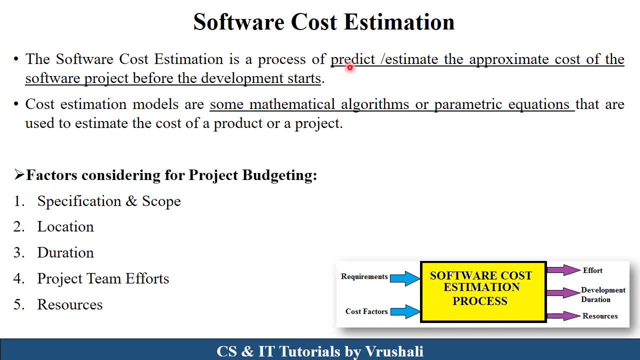 Basically, software cost estimation is a process who predict and calculate total cost required for a project. So in this session we will discuss about software cost estimation. Now for completing a particular software project. this cost estimation process handle in planning phase of software development life cycle. For that purpose they use different mathematical 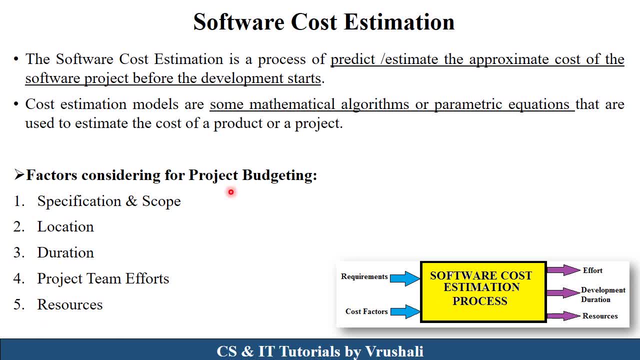 algorithm and different parametric equations. There are different factors which affects on project budget, like specification and scope of particular project, location, duration, different project team and different resources required for completing a particular project. So by analyzing all these factors, we can calculate the cost estimation process. So let's start the session. 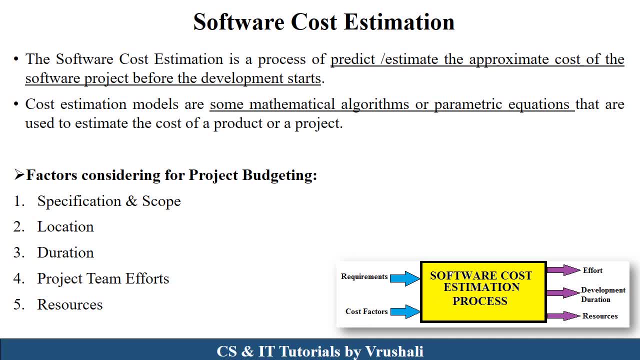 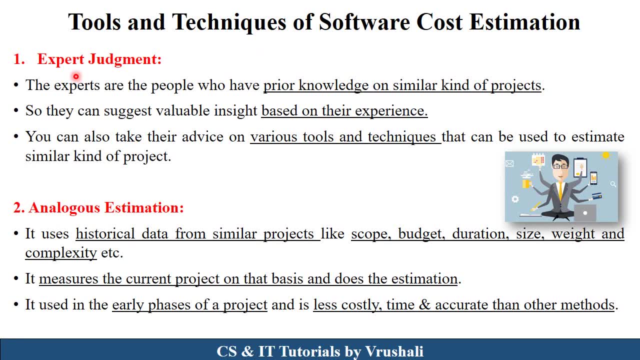 factors project manager decide the cost of particular project. The next point is tools and techniques of software cost estimation. The first technique is expert judgment. See, there are various expert people who have a knowledge of similar kinds of project. So project manager discuss with. 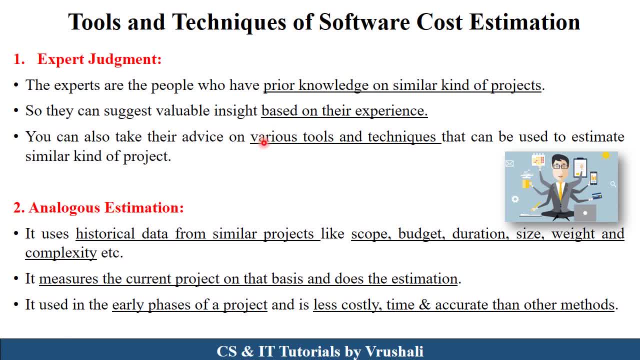 expert that how to decide a software cost, which type of tools and techniques used for estimation the cost of particular project. so expert gives you a suggestion according to their experience. so this is one of the most important technique for decide the cost of particular project. the second technique is analogous estimation. here project manager analyze all the historical project. 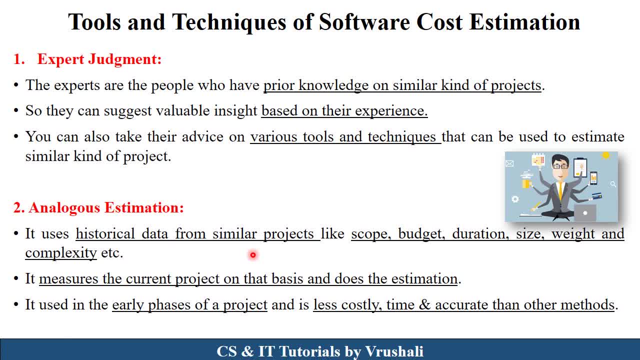 or all the similar type of project that have already developed. project manager analyze scope, budget duration, the size of particular project, the weight and complexity of particular project that have already developed and according to that past project they decide the budget of your current project. so this analogous estimation is a very early phase of particular project. 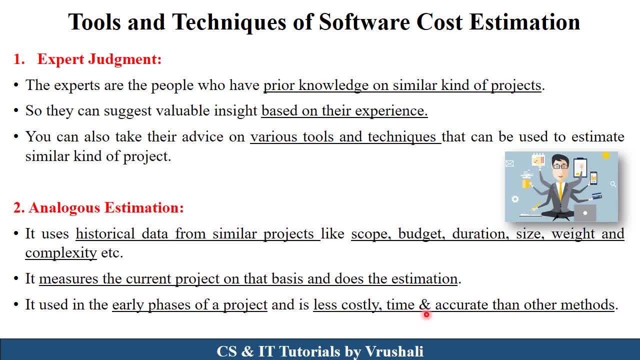 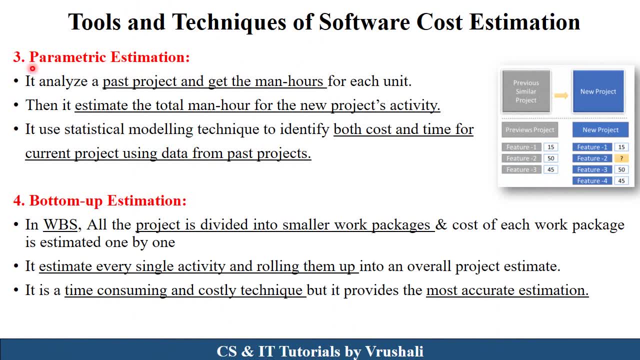 which required less cost, less time, but which is less accurate than other methods. so this is called as analogous estimation. the next technique is parametric equation. here project manager analyze how many human resources or how many manpower required in past project. so according to past project they decide how many man hour or how 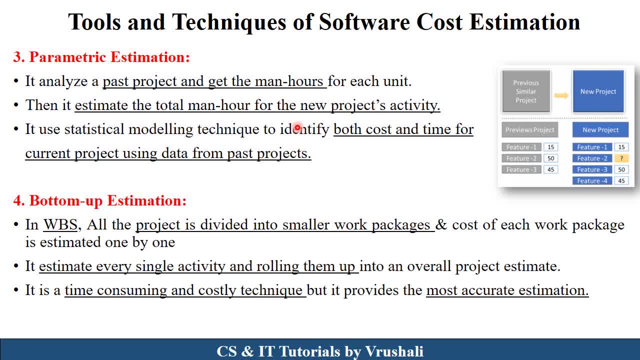 many human resources required in current project. they analyze all the modules activities that generated in past project and according to that they decide all the thing in your current project. this is called as parametric estimation. the next technique is bottom up estimation: see in previous session we discussed work breakdown structure. 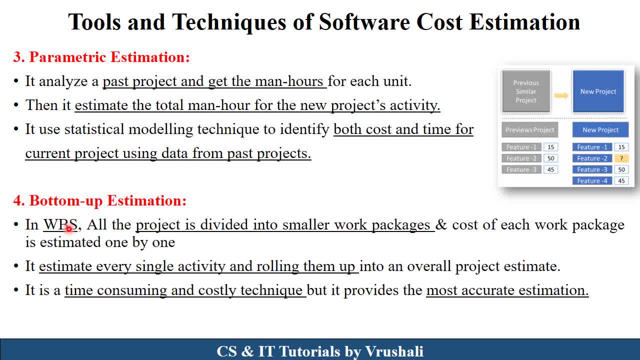 they divide your complete project into the smaller task, right? so due to bottom up estimation, it is very easy and it is very time consuming process to decide a cost of particular activity because in wbs structure there is a division means. suppose there is a requirement gathering, so for requirement gathering purpose there is a interview group discussion, then service gathering. 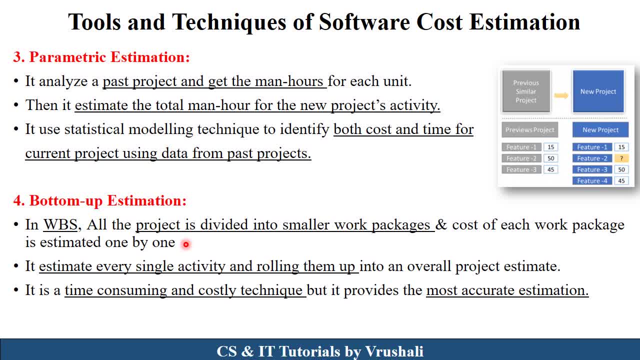 way. so for all this activity, how many cost is required? the next one is a design. so in design there is a structural design, architectural design. so for each design purpose how many cost is required? so this all things have decided in bottom up estimation. they decide the cost as per the wbs. 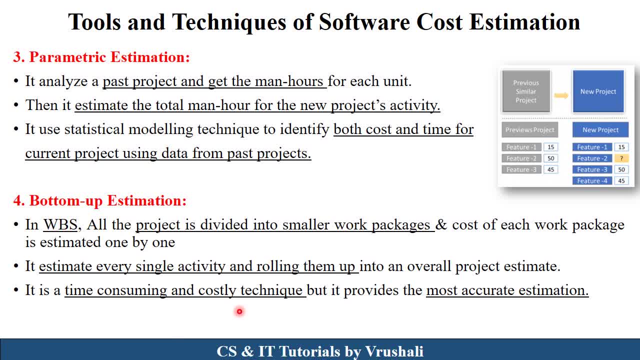 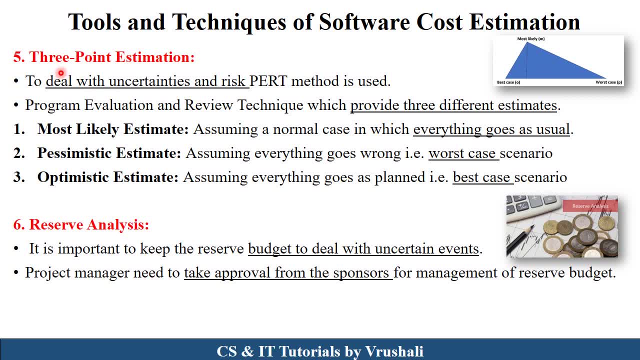 structure. it is very time consuming and costly technique but it provide most accurate estimation. now the next technique is three-part point estimation. see, in your project there are different uncertainties and different risk have generated. so for that purpose, pert, that is, program evaluation and review technique- this method is 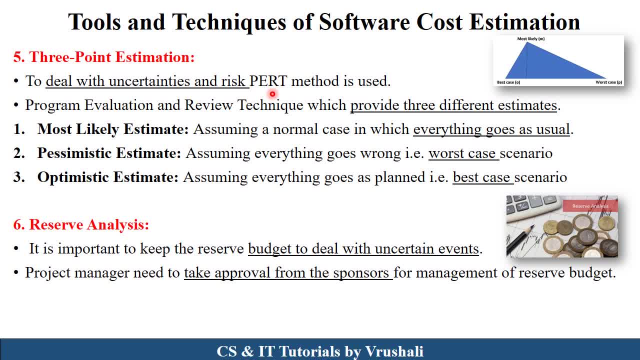 used. we already discussed prt method in previous session. so in prt method they calculate three point. estimation means first they calculate most likely. estimation means everything goes well in your project, then what is the cost of particular project? the second one is a pessimistic estimation. suppose there are various issues, various. 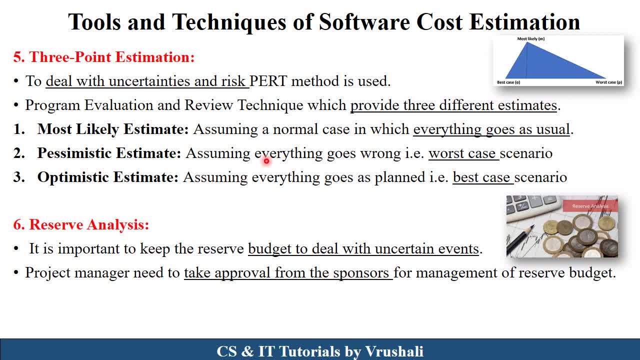 problems have occurred, delay in particular project. then, in worst case scenario, how much cost of particular project? and the next one is a optimistic estimation. so here everything goes well according the planning. so in best case scenario, what is the cost of particular project? they analyze the cost of particular project in three point estimation. the next technique is reserve. 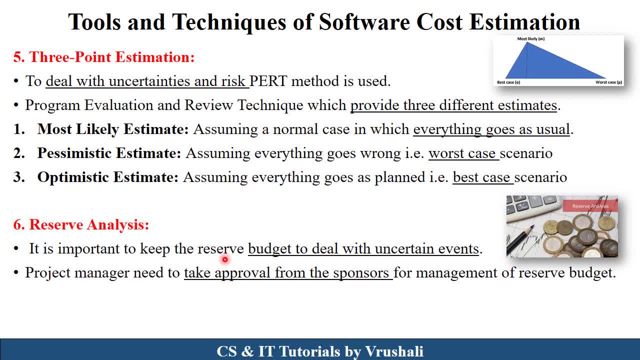 for example, up to this project. so reserve money is cakey and budget for project is absolutely important, right? so reserve budget is usually the most important for every project and therefore place your budget like the basis condition, right? so to study this basic Por Government: short a particular project, you decide the budget. so in this particular case, on your project. but 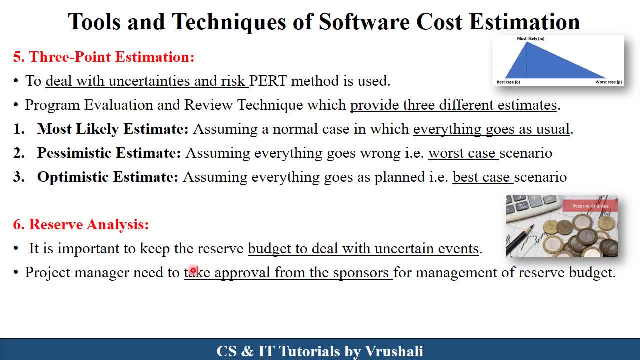 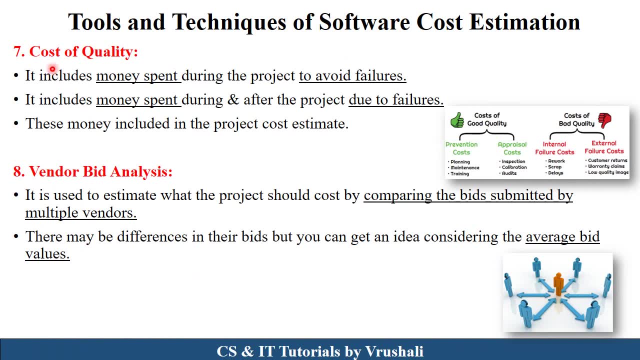 reserve budget is one of the most important reasons you decide the budget for that particular project. so, though, budget is not that fundamental for the project deligibility, you know. labour drivertwice' budget should also have grace and security from those desi money, particular fund for future development purpose. now the next technique is cost of quality. 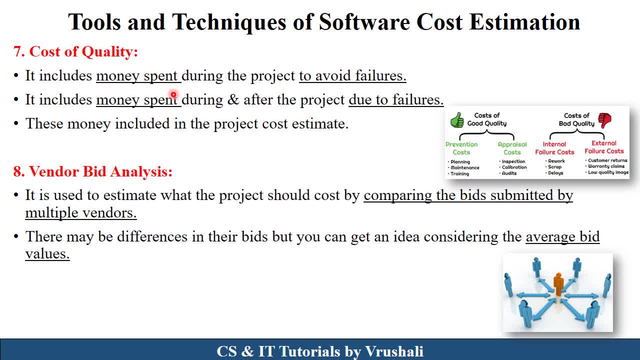 see in particular project money spent on particular project to avoid failures. this is one thing, and the second thing is you can spend money on particular project after failure have occurred, right. so this is called as cost of quality. see here: cost of good quality means you can reserve. 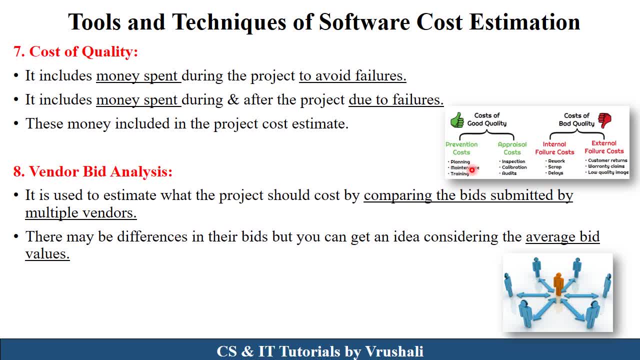 money, or you can spend money on planning phase, maintenance phase for training phase than a different collaboration and inspection phases. so it is a good quality money. but when you spend money on, when your project get delay, low quality images are there, customer returns are there. so for that, 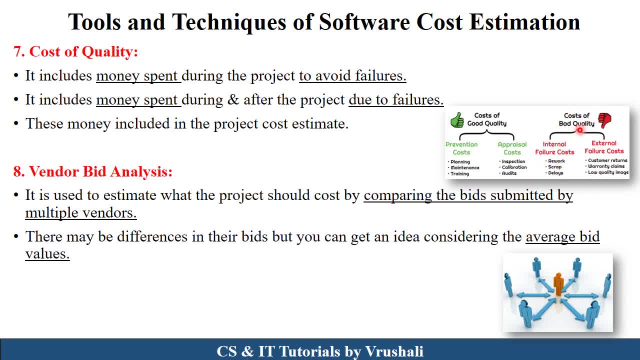 purpose. when you spend money, this is called as cost of bad quality. so this money also included in the project cost estimation. to decide: project manager: decides to spend money on project cost estimation, so this money also included in the project cost. decide this thing: which is a good quality cost and which is a bad quality cost, then 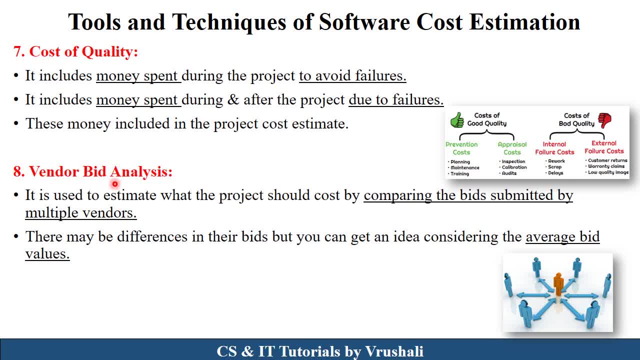 the last technique of software cost estimation is vendor bid analysis. so in particular project there are different software and hardware resources are purchased right, so there are different vendors for that purpose. so project manager buy a particular hardware for particular vendor. at that time project manager compare price of multiple vendors. the cost of particular. 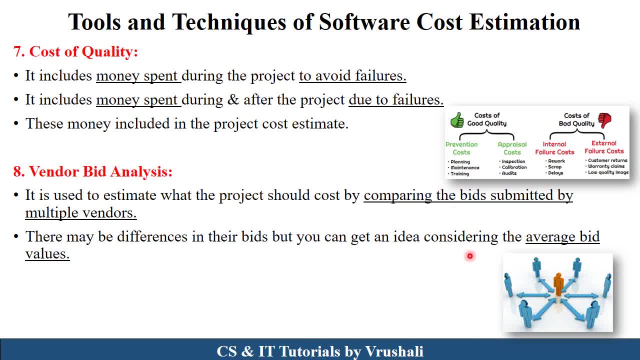 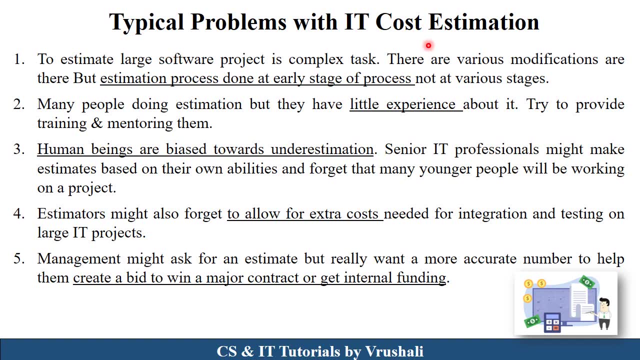 hardware from multiple vendors. so at that time project manager decide the average cost of particular hardware from particular vendor. this is called as vendor bid analysis. now the next point is: various problems occur in it cost estimation. see as we discussed earlier. software cost estimation: decide at early stage. 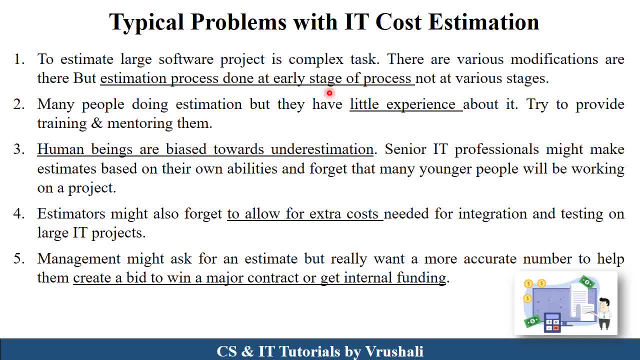 of process means before start the development. but what happen after development? there are some issues and problems have occur. so at that time, modification of cost, it is very difficult. so this is one of the most important problem. second time, sometime many people doing the estimation, but they have a not much experience. they have a little experience in that. so always, 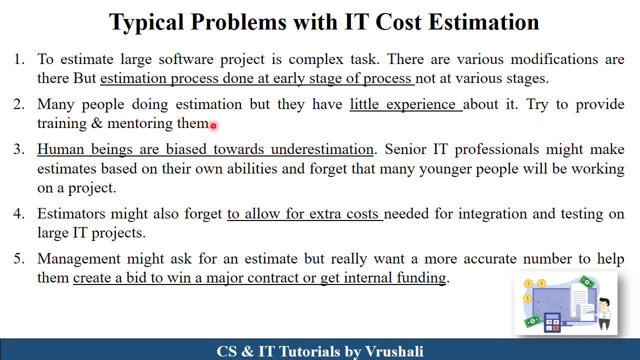 try to provide training and mentoring all the people who estimate the cost of particular project- Number 3.. The third problem is human beings are biased toward undetermination. see, in particular project there are various senior IT professionals and also junior IT professionals, So decide the cost of particular employee and particular human resources is get difficult. 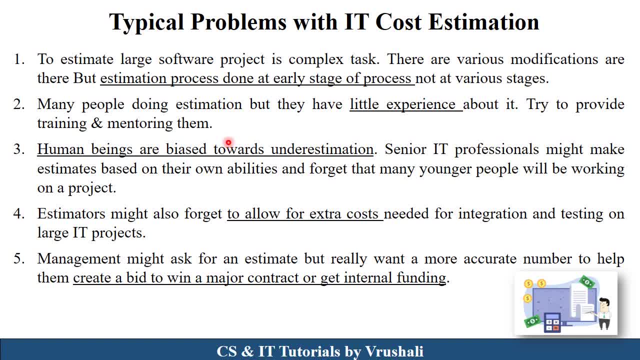 because they have some abilities, some skills. So there are some bias toward undetermination in particular project. The second, the next problem is: sometime what happened in particular project? they got extra cost means in testing. there is a integration testing, unit testing, then black boss testing system testing. different types of testings are there. 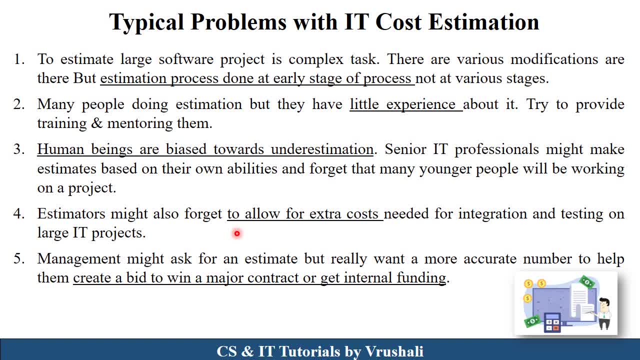 So sometime it required extra cost in particular project. So this thing also decided in early stage of process. So which is not a good thing. And the last thing is sometimes what happened. there are various vendors in particular project. So to compare all the vendors, to compare all the price of particular hardware resources. 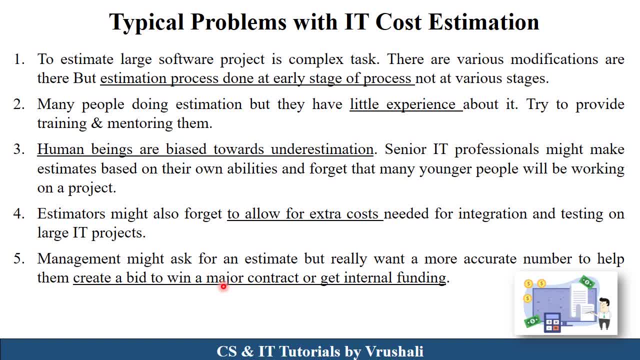 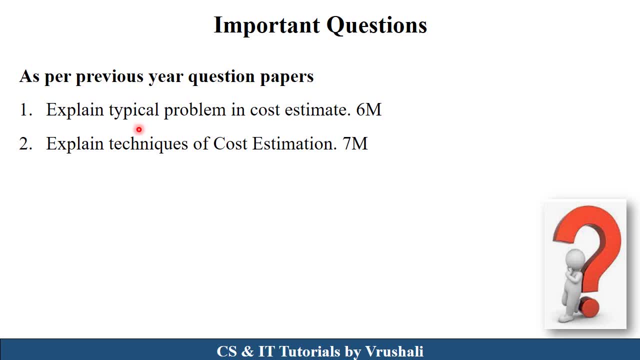 it is very difficult thing. So that's why they provide a particular training and mentor, the particular person who analyze all the cost estimation. So these are the different problems occur in IT cost estimation. Now, as per your previous year question paper, these two are the important question, like 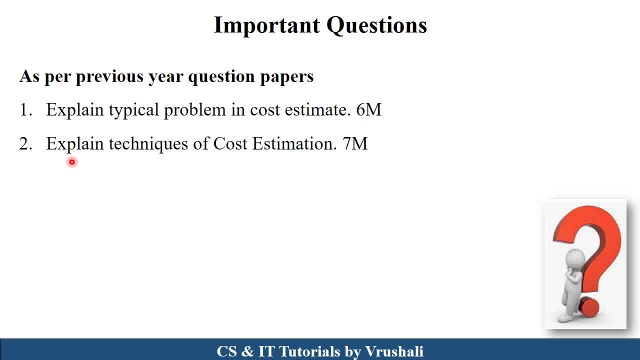 explain typical problem in cost estimation for six marks and explain techniques of cost estimation For seven marks. from these two question, the first question is most important. So thank you, Keep learning.